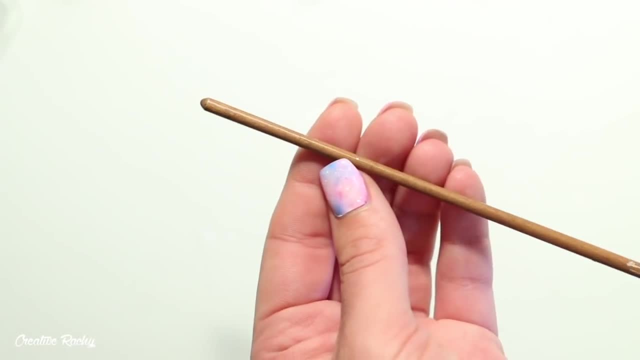 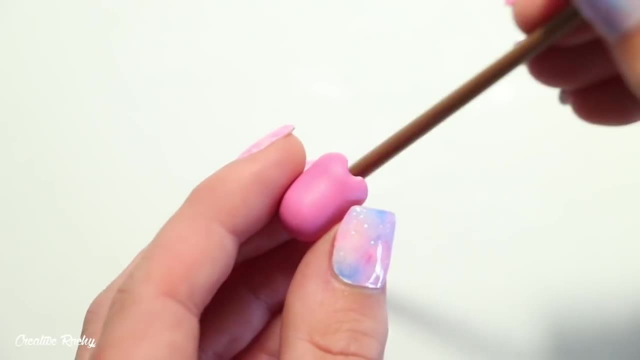 So, once you've made the body shape, it's time to create the legs. For this, I'm taking a paintbrush and I'm going to be using the handle, but you could use any other tools that you would like. I just pressed the handle into one end to make an indent, which creates the two legs. 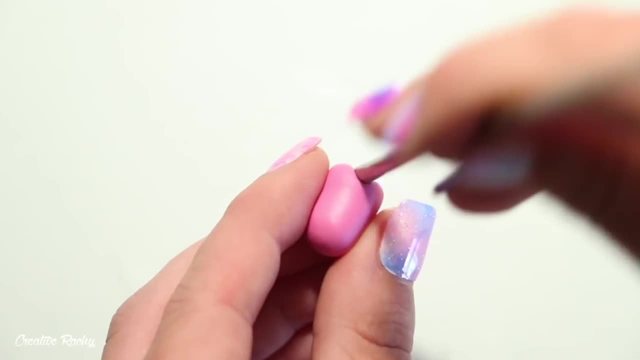 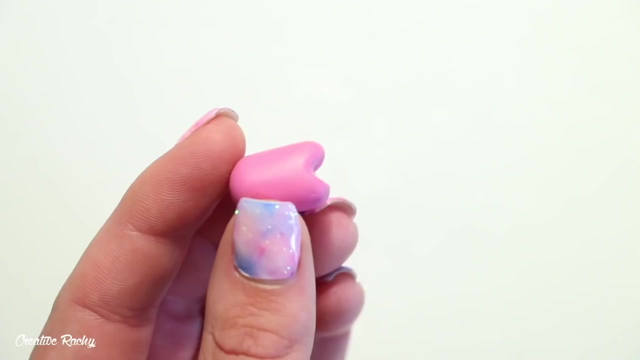 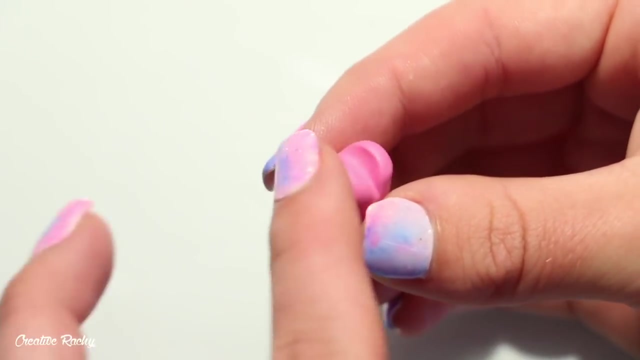 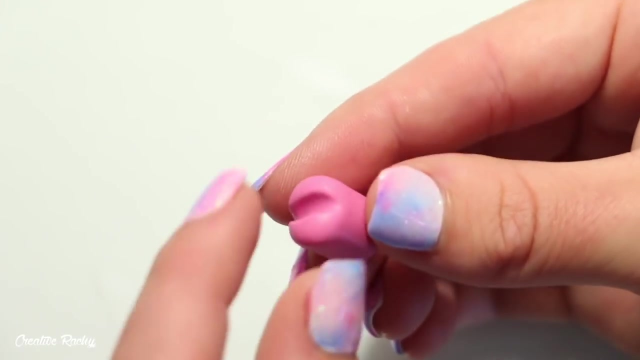 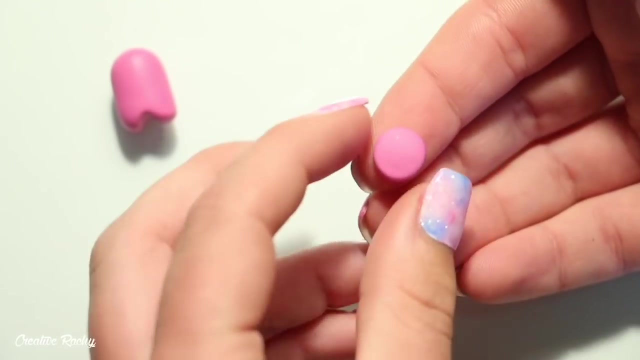 And then, as you can see, the lines are still quite harsh, so I went ahead and smoothed it out with my fingers to make them more rounded. Next, I'm going to do a- So this is what the body currently looks like. To make the oxygen pack or tank, take some more clay the same colour as the body, and you'll want to shape this into a little square. 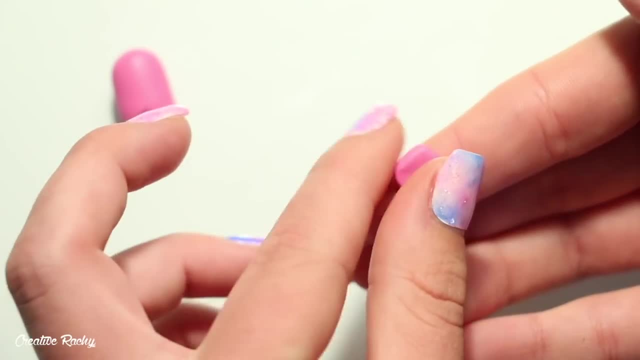 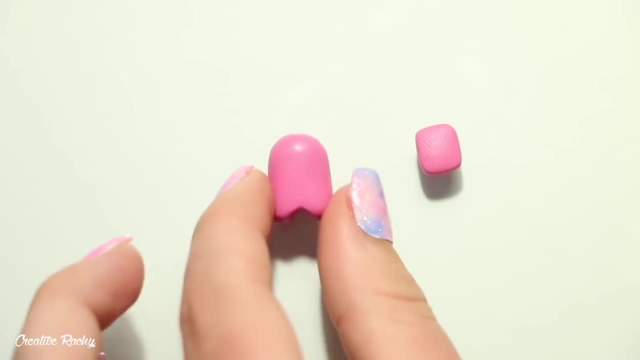 So I've got a little square here and I'm going to shape it into a little square. firstly flattened my clay down and then I pushed in the sides to make them straight. You can then flip over your character and position the pack onto the body. 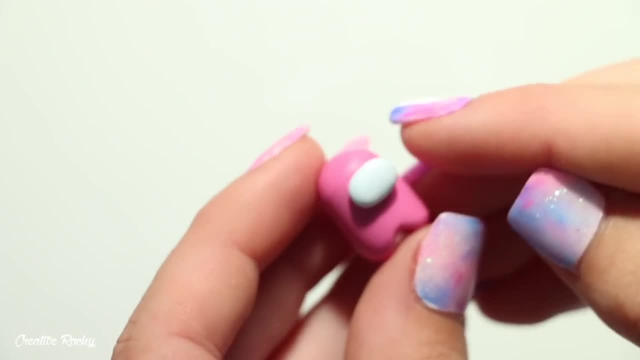 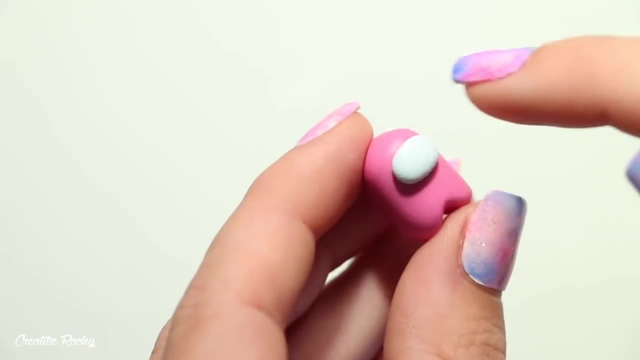 Now to make the eyepiece or helmet, you want to take some light blue clay and shape it into an oval, and then you can just go ahead and position this onto the front of the character For extra details. here I'm adding the little light reflections and shadows. 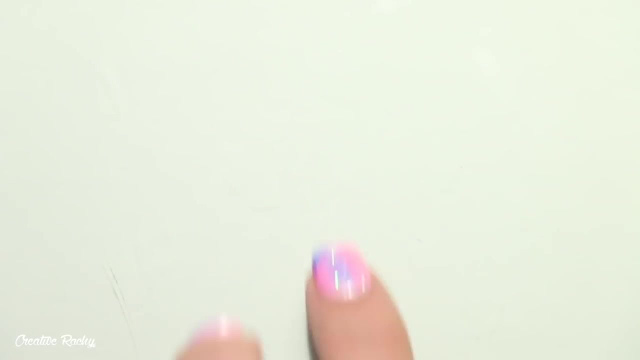 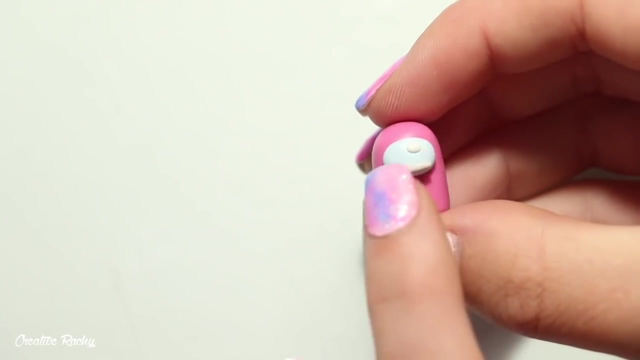 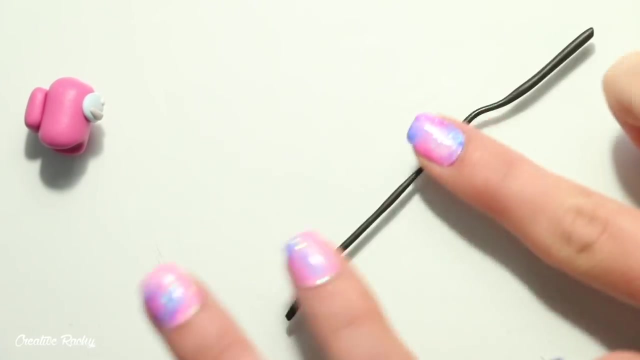 so for the light reflection, I attached on a small ball of white clay to the top part of the helmet and then I also rolled a coil of some grey polymer clay and I attached this onto the bottom of the helmet for the shadow. To finish off, we are going to add a black rim around the outside, so roll a coil of black clay. 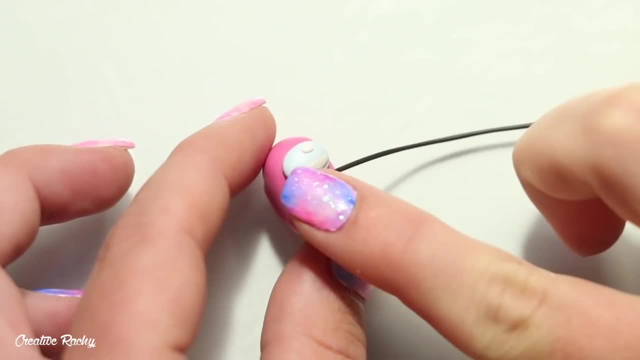 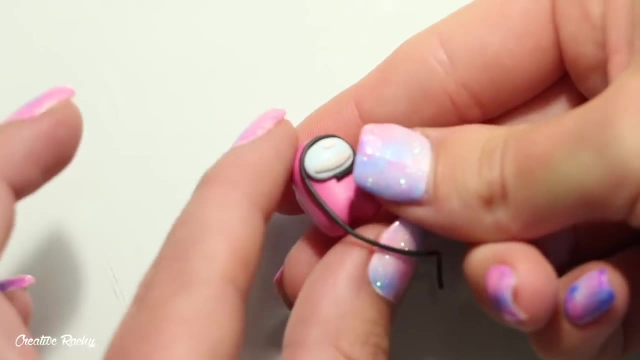 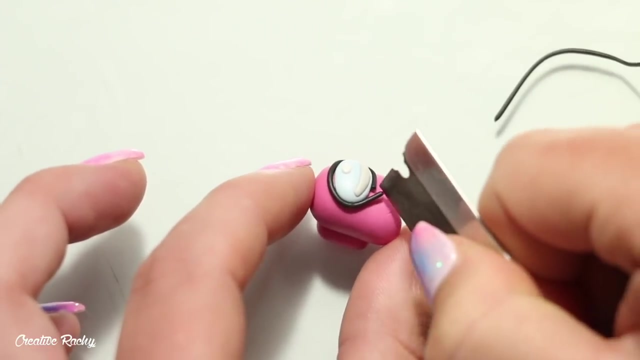 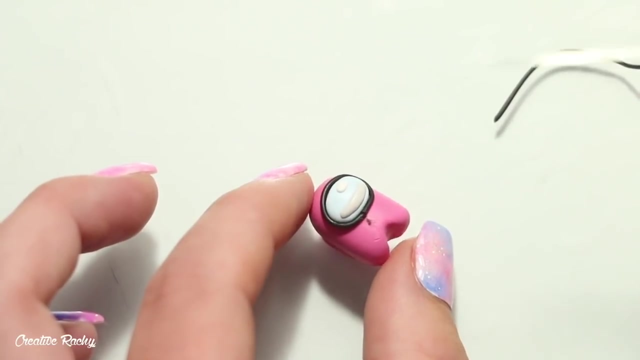 on your work surface and then roll it onto the top of the helmet. Then you can very carefully wrap this around the helmet and cut off any excess clay that you have. Here you can see that I accidentally pushed some of the black clay onto the body, so here I'm just 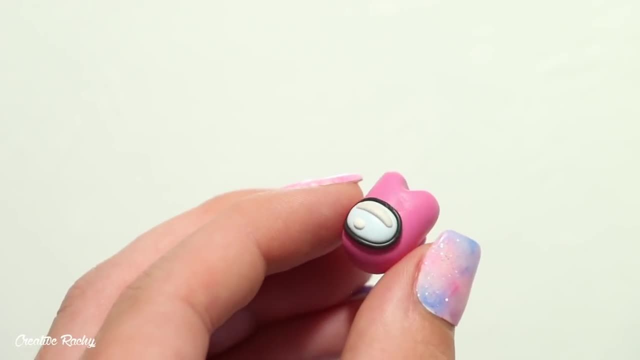 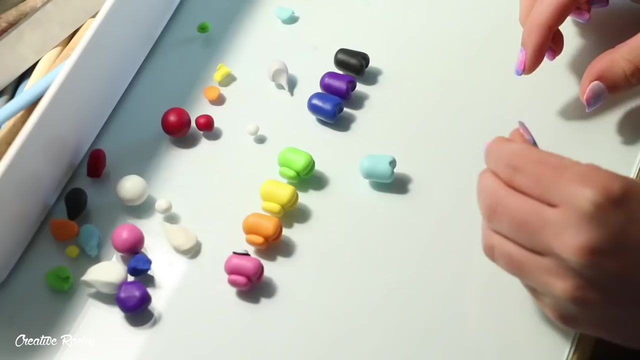 very carefully, scraping it off with a blade. So I just then went ahead and cut off the excess clay that I had on the helmet, and then I just went ahead and repeated these same steps with my other colors for the other crewmates, and here's just a quick time lapse of me doing that before I show you how to make the different. 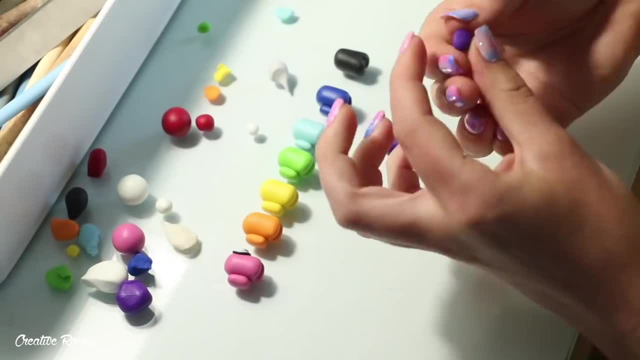 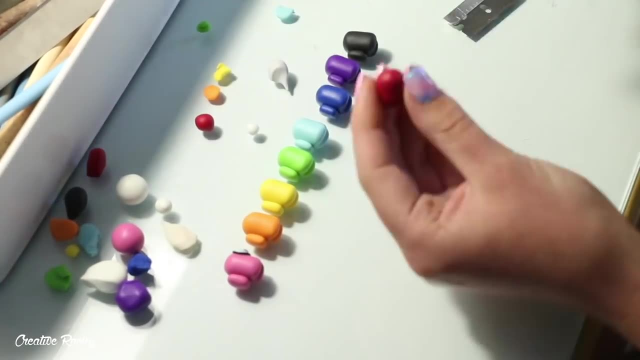 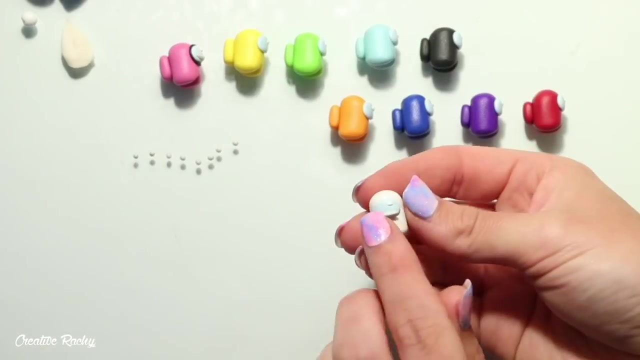 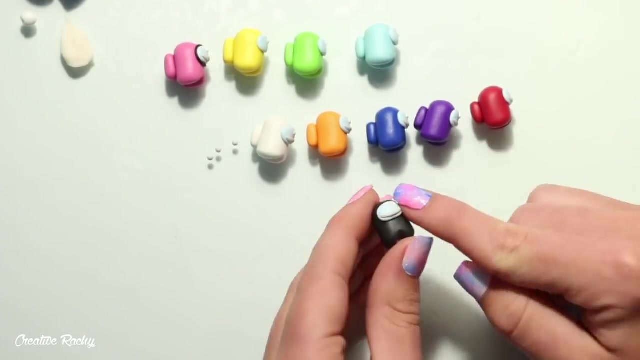 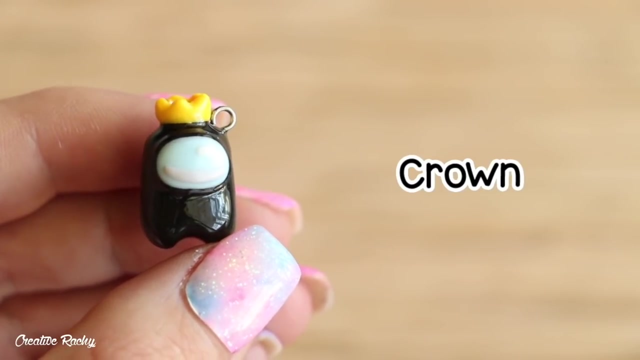 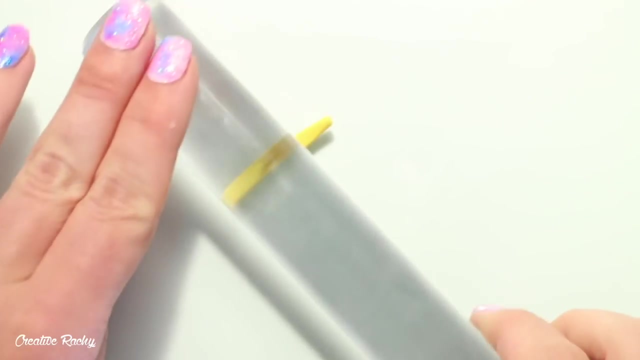 designs of hats. So I folks have 34 colors, so you can do a set of your own what you think your now have. For this you want to use some yellow polymer clay and I started off with a small ball which I rolled on my work surface to create a coil. 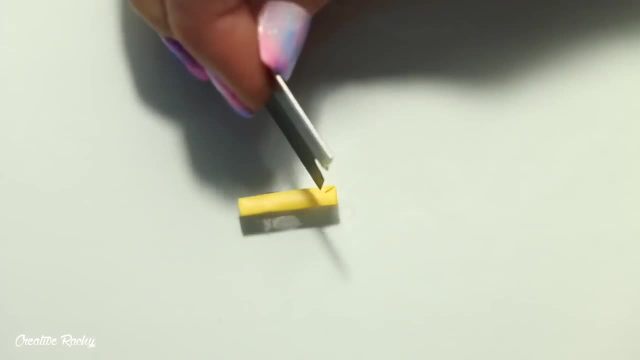 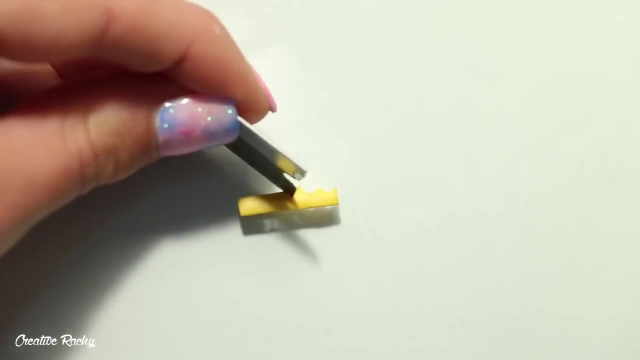 Next, use a rolling pin to roll and flatten down this coil. You'll want to trim off the ends and also one side of the clay so that you have a straight edge, and cut out some triangles using your blade. i just kept going along until i got all the way to the end. 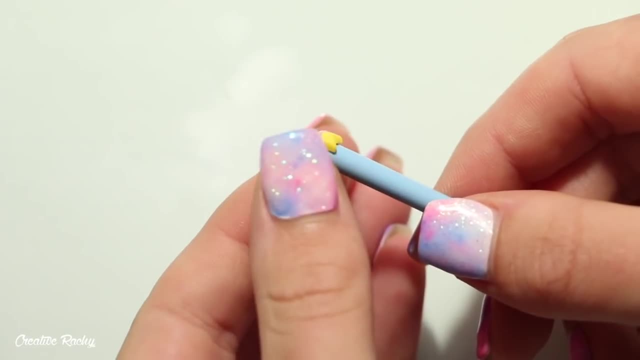 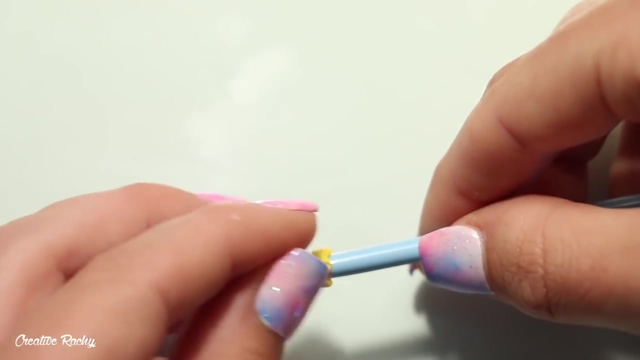 i then wrapped this clay around the handle of one of my tools, which i thought was a good size, and this just helped me to get the round shape of the crown. i kind of pinched the ends together with my fingers to try and blend them, and then i very carefully removed the crown from the handle and placed it on top of the character. 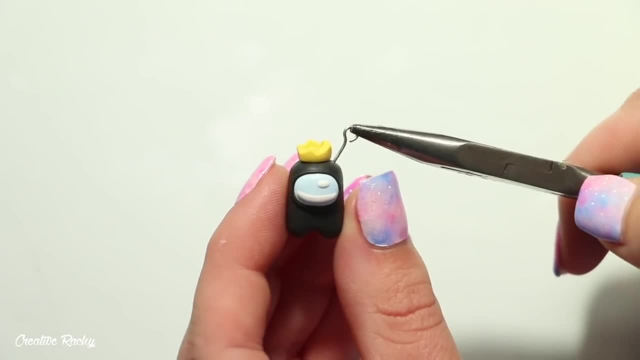 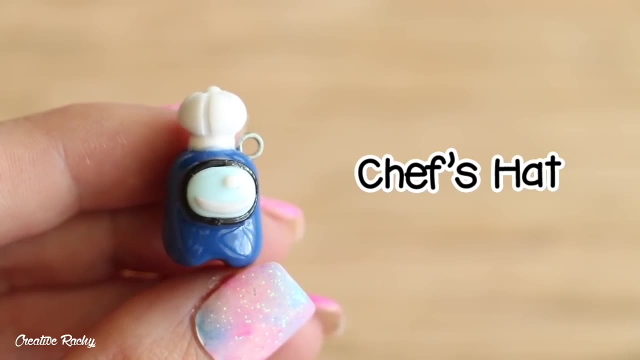 if you would like to make it into a charm, go ahead and add an eye pin, and then you can bake it in your oven according to your package's instructions. next up, we are going to be making the chef's hat. to begin, i took two balls of white clay. i firstly took the large one and i began. 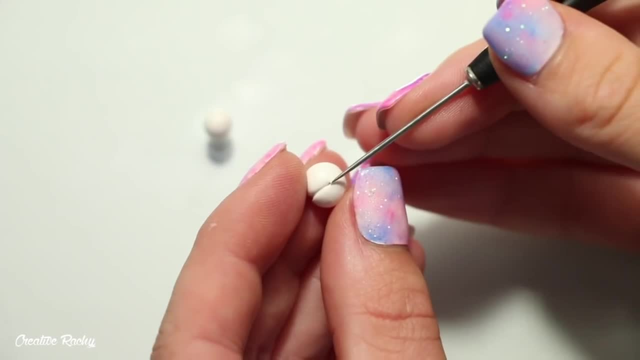 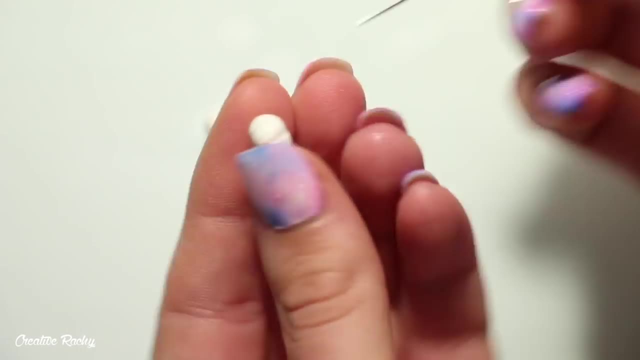 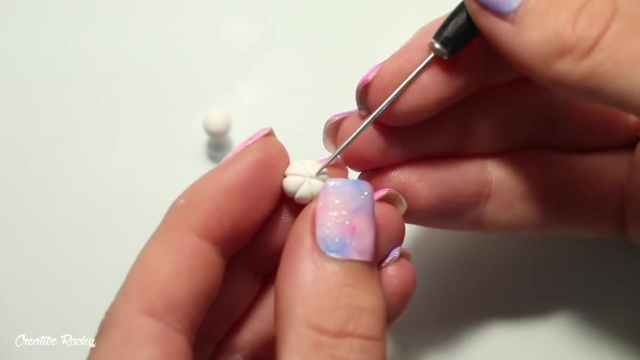 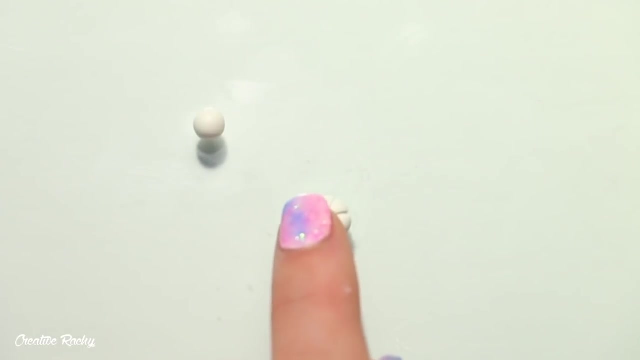 adding some indents using my needle tool, almost so that it looked like a little miniature pumpkin. i then created an indent in the center using a dotting tool and i placed in a small ball of white clay for the little button where the fabric meets. i then took the other piece of white clay. 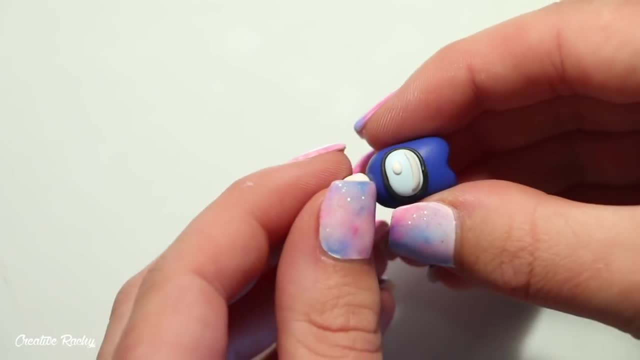 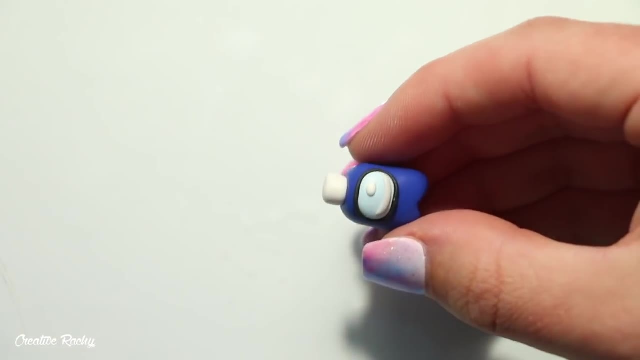 that i had at the beginning and i rolled it into a cylinder which i positioned on the top of the head and i pushed down. then to this i added the top of the chef's hat and i made sure that it was centered, and i then added some more white clay to the center to make it look like a little. 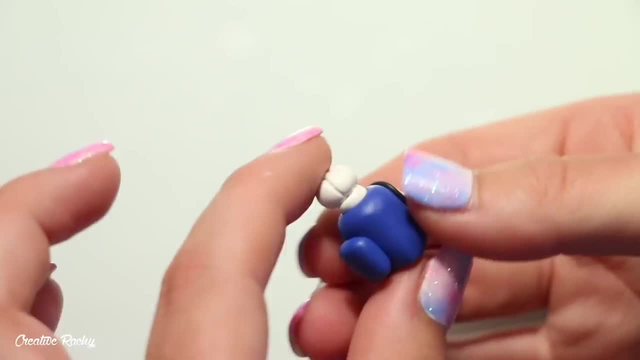 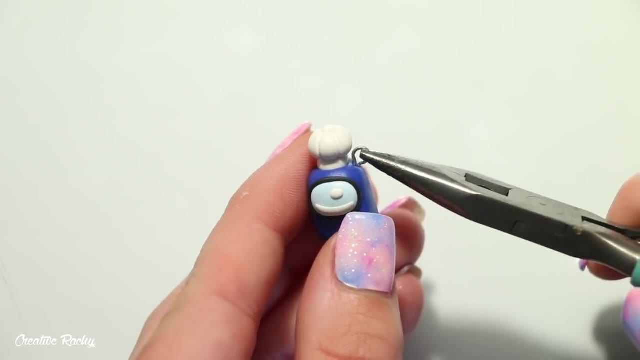 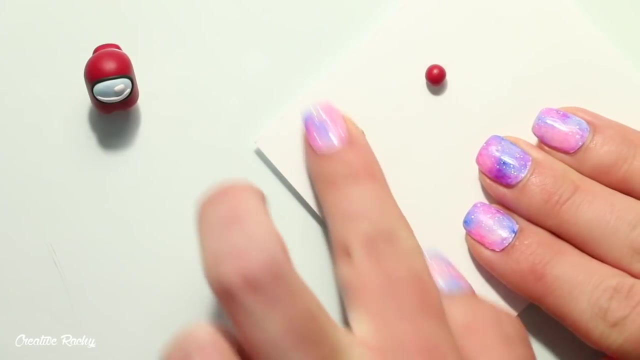 mushroom and looking okay, before then adding my eye pin to make it into a charm and baking it in the oven. next up, we have the devil's horns, and i'm going to be doing this on the red crewmate. so i began with two balls of red clay and i rolled these down into teardrops. 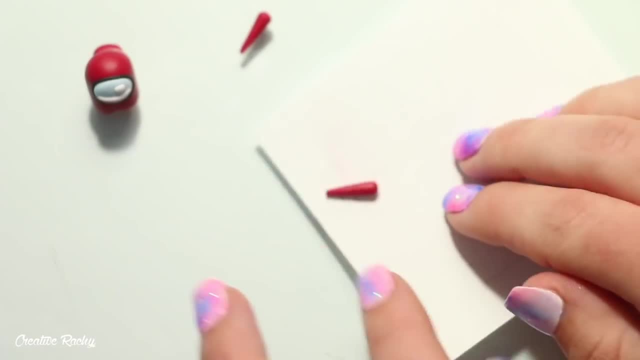 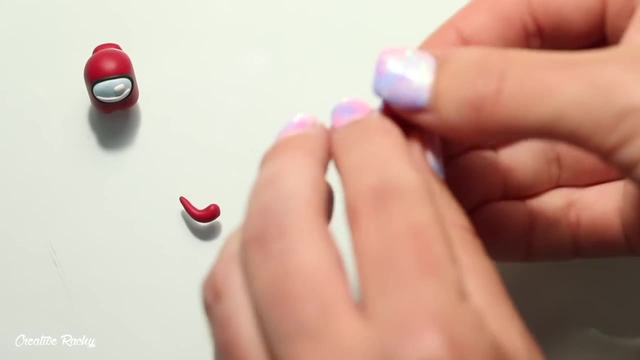 here. you can see that i'm doing this on a sheet of paper because there's more friction and i wanted to prevent the clay from slipping around on my work surface. Once I had created the teardrops, I then bent the clay so that each one had a curve, Then use your blade to trim off the rounded part. so 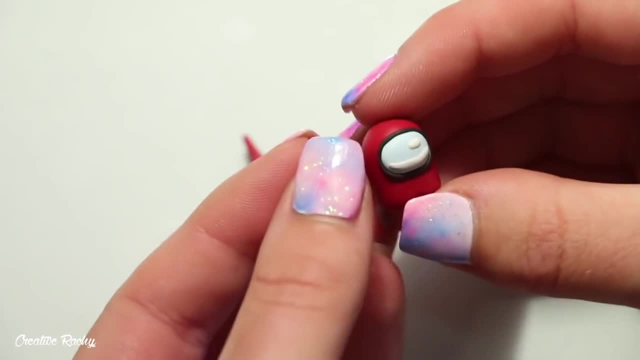 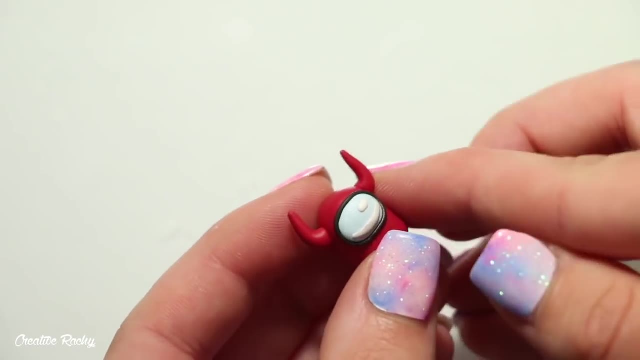 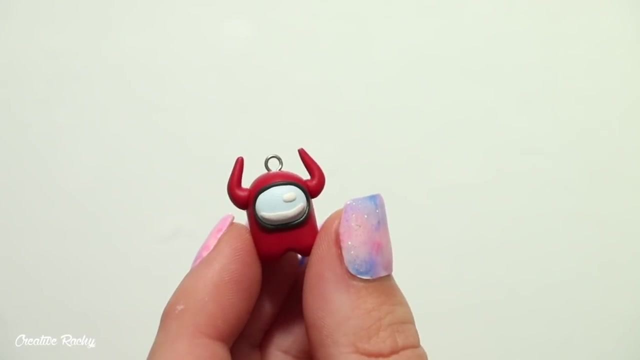 that you have a flat surface to work with, and then you can go ahead and position these onto either side of the head, Add an eye pin if you would like to make it into a charm, and then you can bake it according to your package's instructions. Next up, we are making the plant hat, and this is the skin I usually 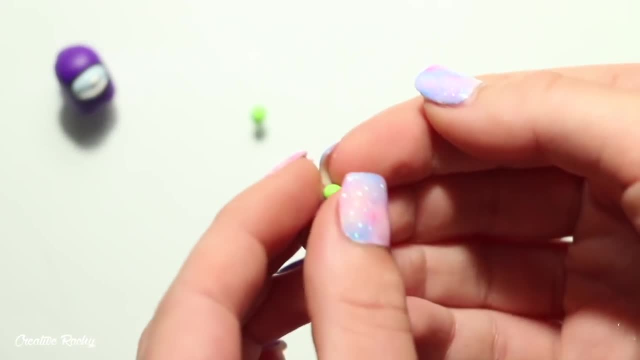 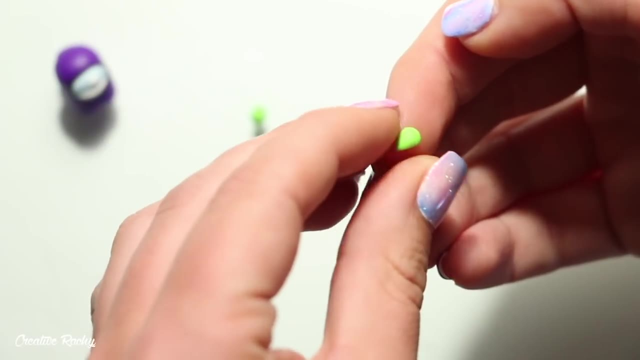 use the purple crewmate with the plant hat, just in case you're wondering. So we begin with two balls of green clay and you want to take each one and flatten it down and then pinch one side to create a tear drop or a leaf shape. I then used my 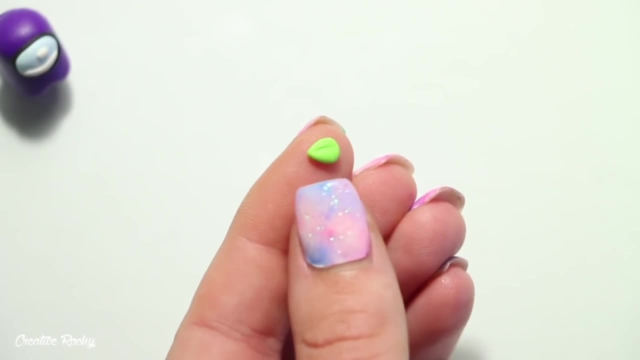 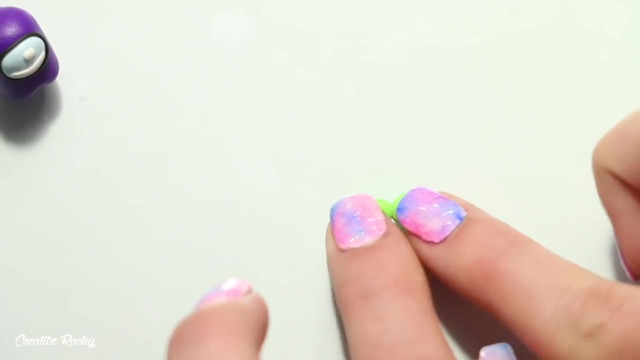 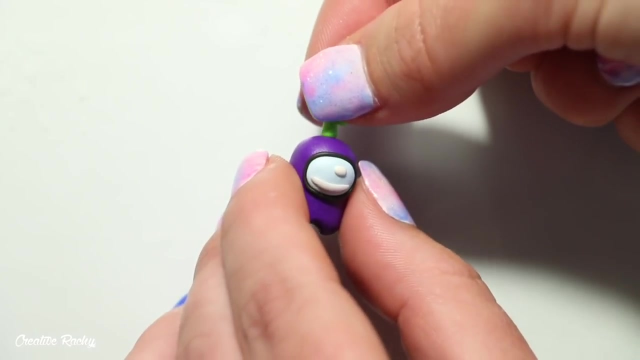 needle tool to create an indent straight down the center of the leaf, and I did this with each of the balls of clay. You then want to position these either side of one another, and then you can add the little stemmed the head before also attaching on the leaves. 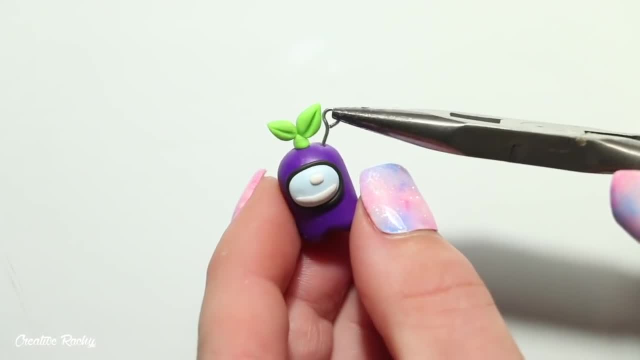 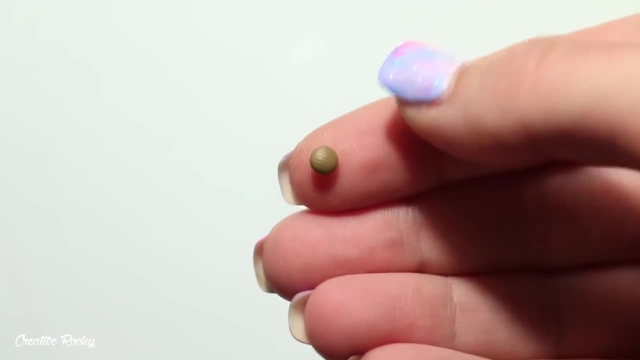 Don't forget to add an eye pin if you would like to make it into a charm and then bake it in your oven according to your package's instructions. The next one we're going to be making is the bear hat, or bear ears. So, to start off, I took a small ball of brown clay, which I pushed down and pinched on one. 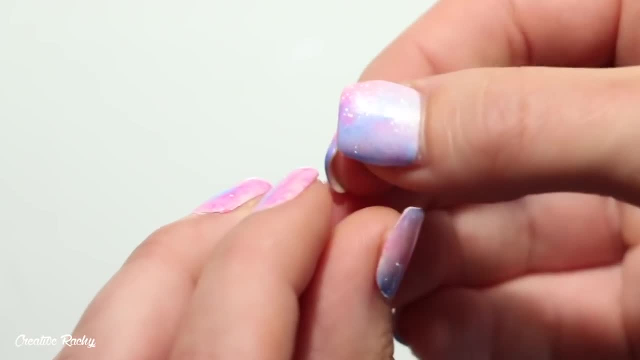 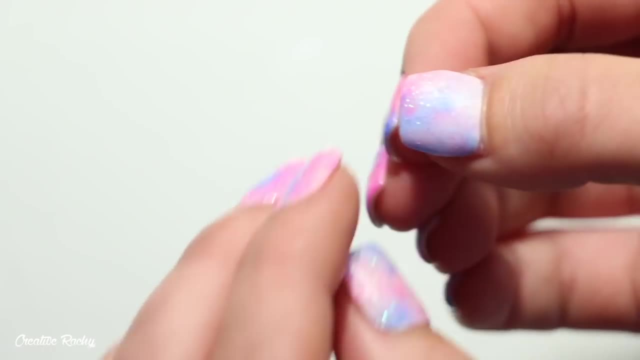 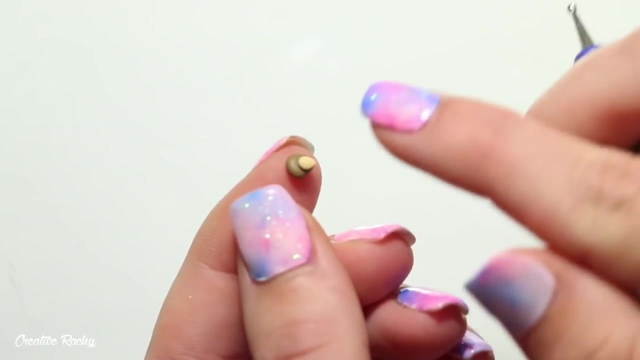 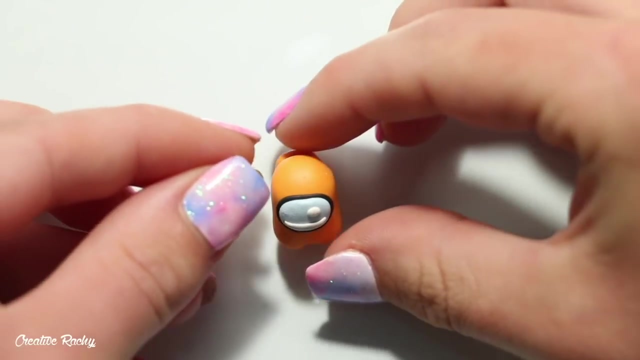 side, similar to the leaf, because you want to make a little teardrop shape. I then did the exact same thing to a smaller piece of tan coloured clay, which I then positioned on top of the brown clay. Next, using your blade, cut off the pointed end, this time so that you have a flat surface. 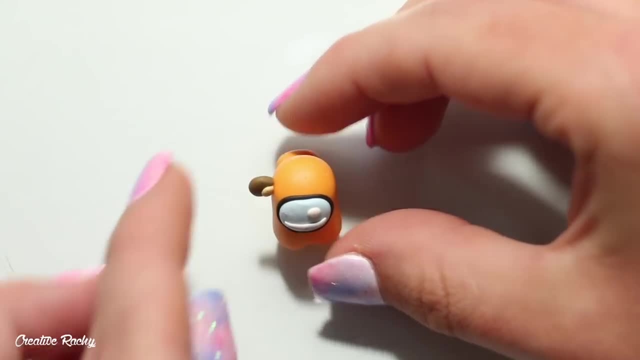 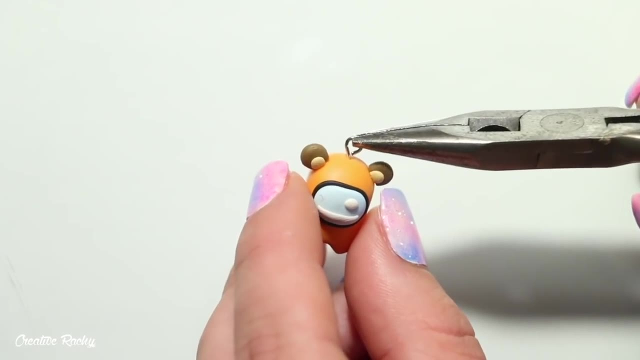 to work with, and you want to make two of these. Once you've done that, you can then position the ears, Add an eye pin to make it into a charm, and then you can bake it in your oven. This next one I'm showing you how to make is the flower hat which I'm going to be placing. 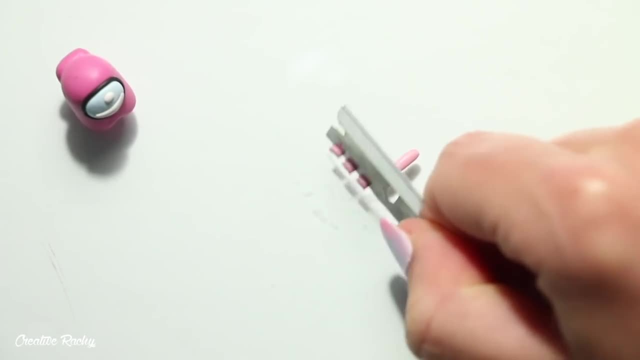 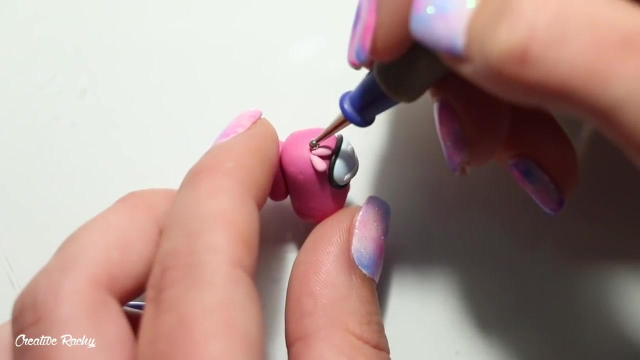 on the pink crewmate. So I firstly began with a coil of light pink clay and then, using my blade, I cut off five even sections, and these are going to become the flower's petals. I shaped each of the petals into that teardrop shape again, and then I began placing them. 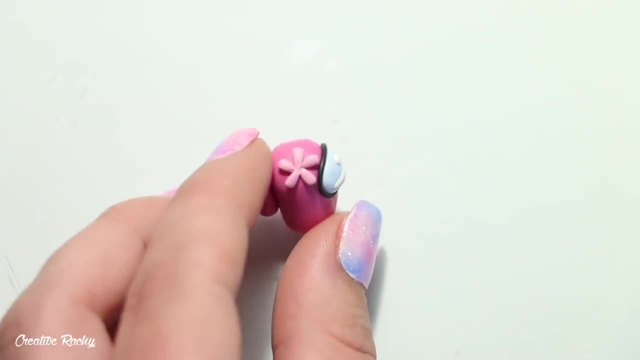 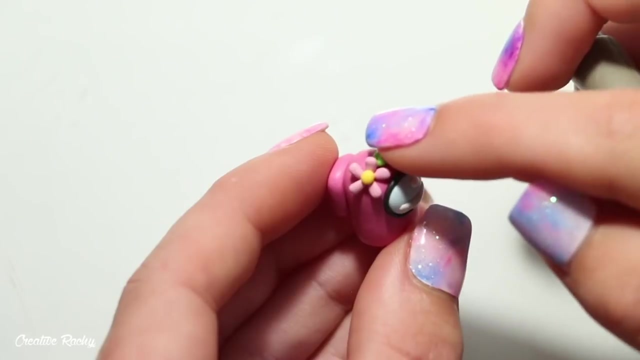 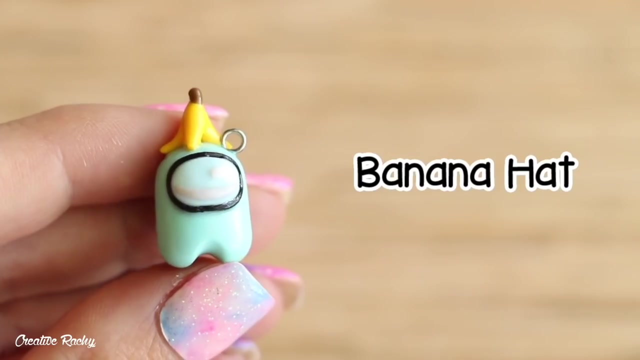 onto the head in a flower shape. I added a small ball of yellow clay to the centre and then on one side I also attached on a little green leaf. Add an eye pin, if you'd like to make it into a charm, and then you can bake it in your oven. 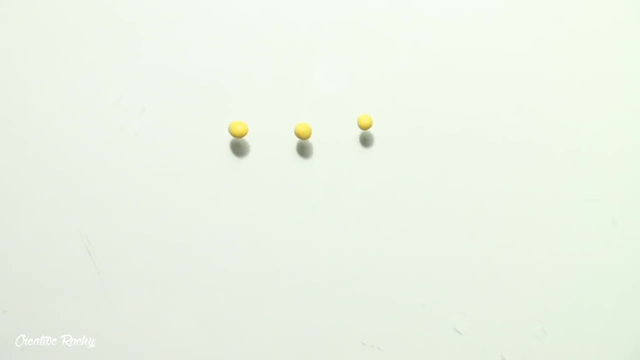 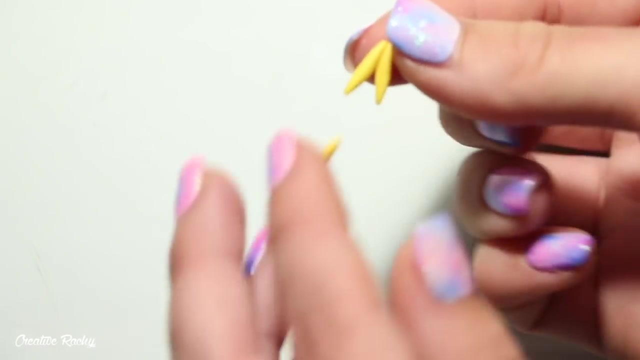 Next up we have the banana hat, which is pretty much just a banana peel. So start off with three balls of yellow clay and roll each of them down into a coil which has pointed ends. You'll also want to flatten these down slightly. Next we're going to attach them all together to make our banana shape. 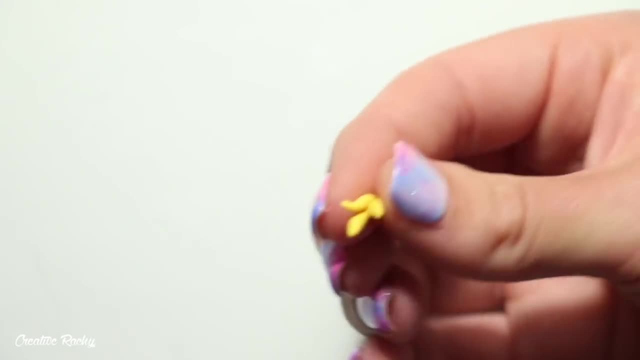 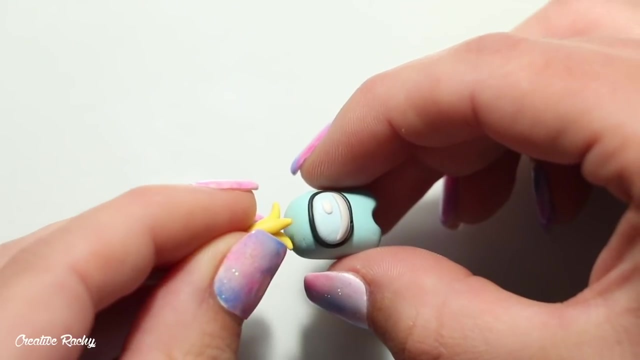 I then roll this very gently between my fingers to smooth it out and blend the joints. You can then curl out the very end of each banana peel and then position this onto your crewmate's head. So there you have it. I hope you enjoyed this tutorial. 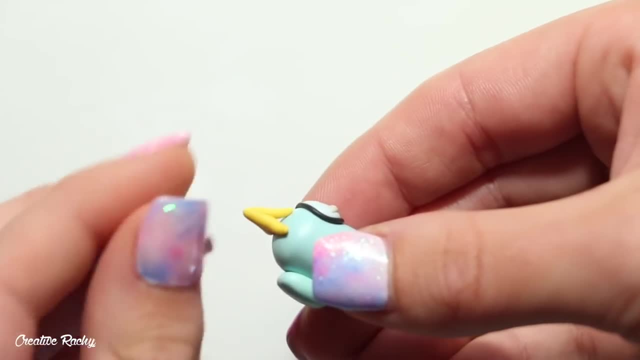 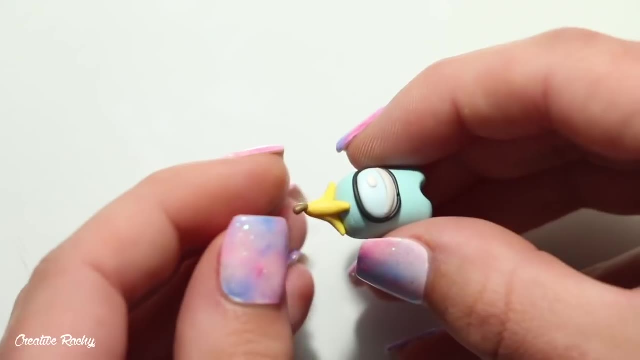 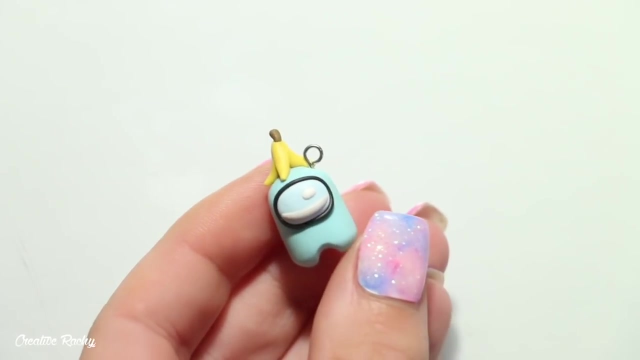 I'll see you in the next one. Bye. For an extra detail, I took a small piece of brown clay and attached it on for the stalk or the stem, and then I went ahead and added an eye pin and baked it in the oven. Now we're going to be making the crewmate hat on a white crewmate, and I guess this design 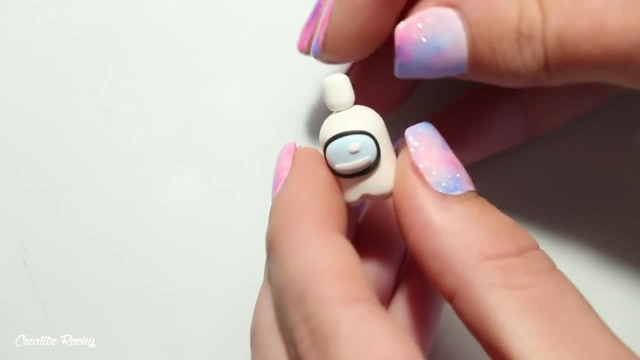 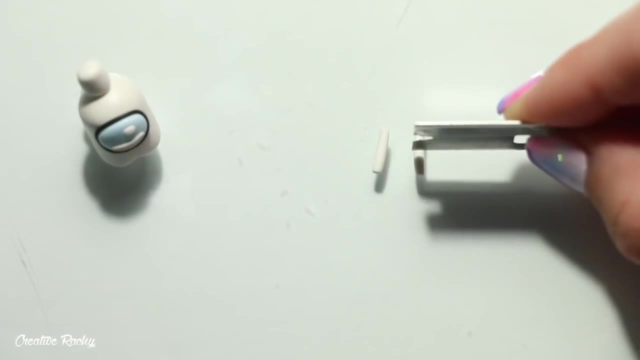 is kind of inspired by the skin that James Charles usually uses when he plays Among Us. So I firstly started off with a little cylinder of white clay which I attached to the head. I then made the legs by rolling out two thin coils of clay, and then I cut off a piece and 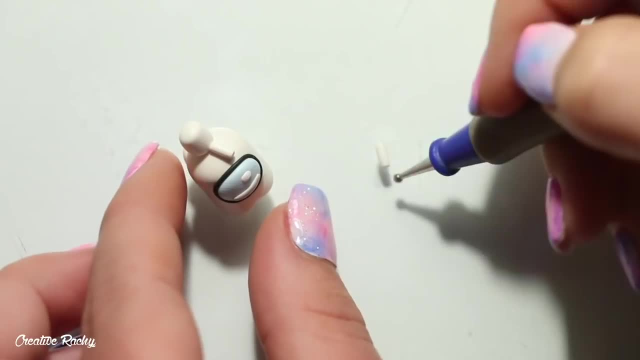 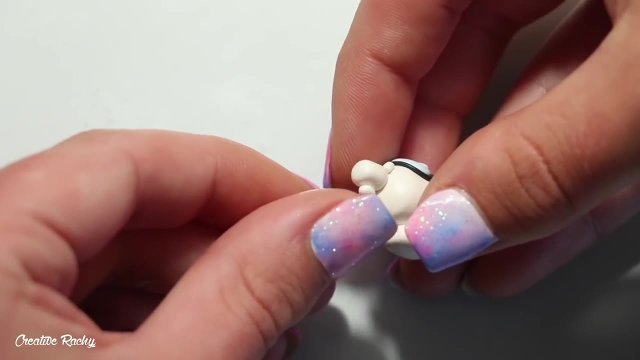 attached these to the little body, kind of hanging them over the crewmate's face. The ones that I'm showing here I found were actually too long, so I removed them in the end and made them slightly shorter. Add a tiny little backpack onto the back of the crewmate's body, and then you can also. 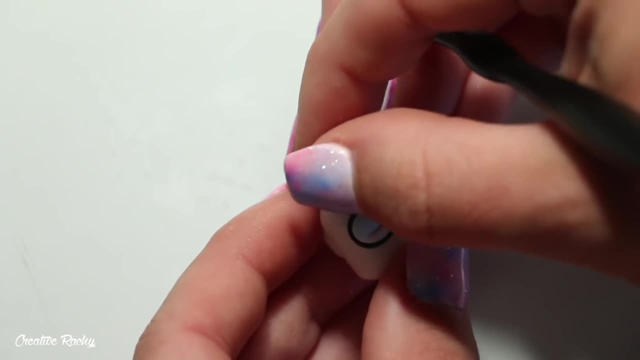 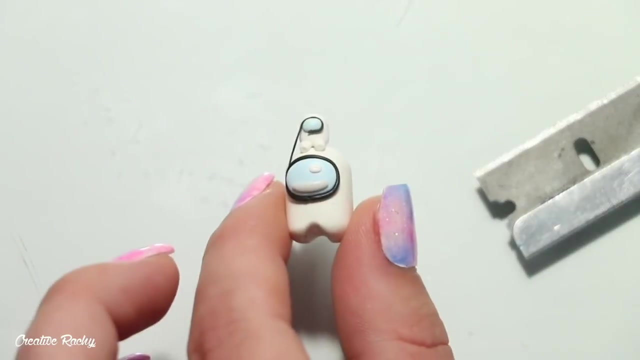 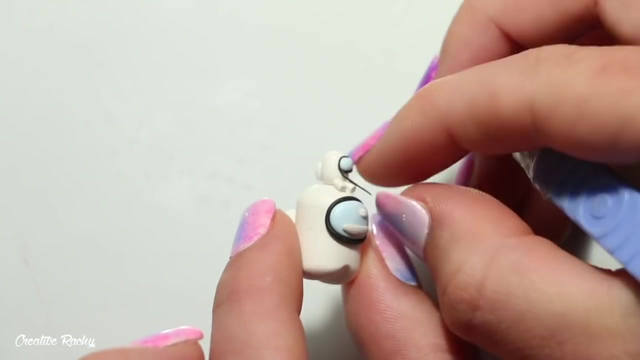 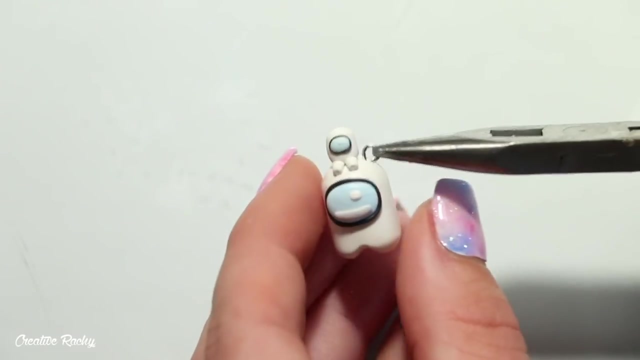 attach on a small piece of blue clay for the helmet and a thin strip of black clay around the helmet for the rim. So there you have it. Add an eye pin to make it into a charm, and then you can bake it in your oven. 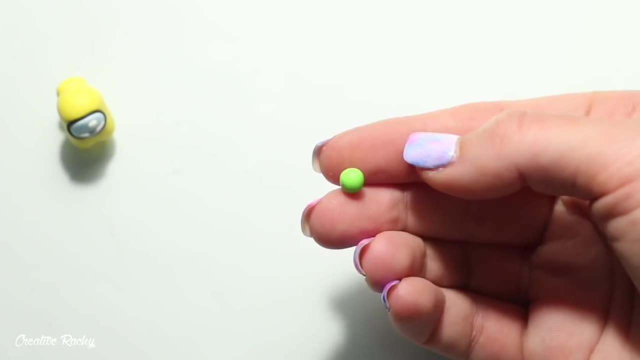 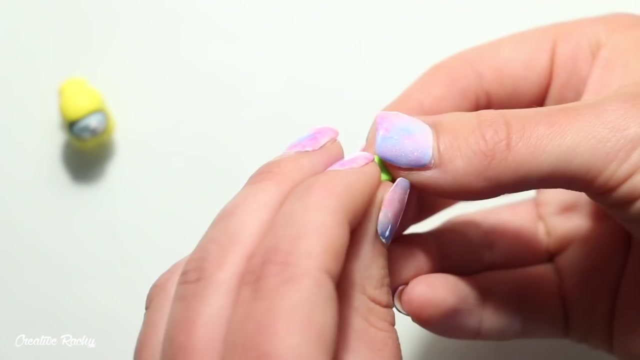 Next up is the brain slug hat, which kind of looks like a little green alien. Start off with a ball of green polymer clay and roll it on your work surface so that it's more of an oval shape To make the legs or tentacles of the slug. what I did was I pinched the clay and kind. 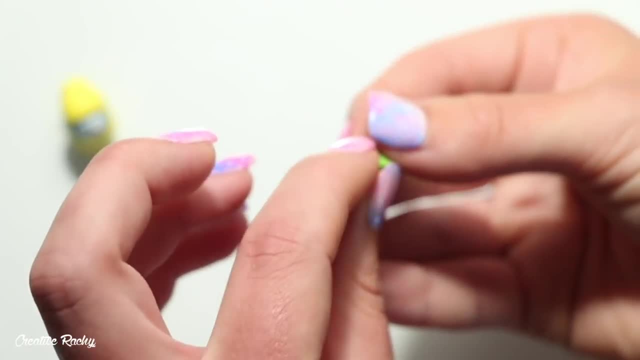 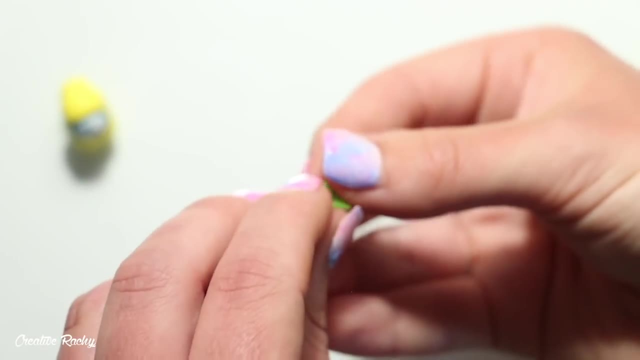 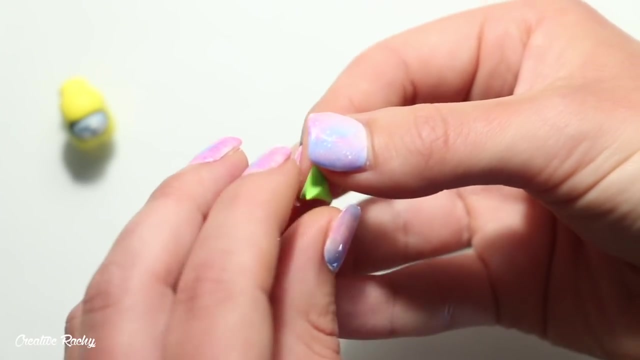 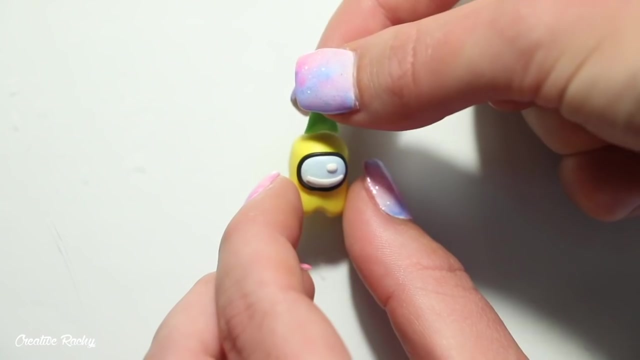 of pulled on it and I just kept going around to perfect the shape until I had three even sized tentacles. You then want to add this onto your crewmate's head, And then you can perfect the shape a little bit more, as you would like. 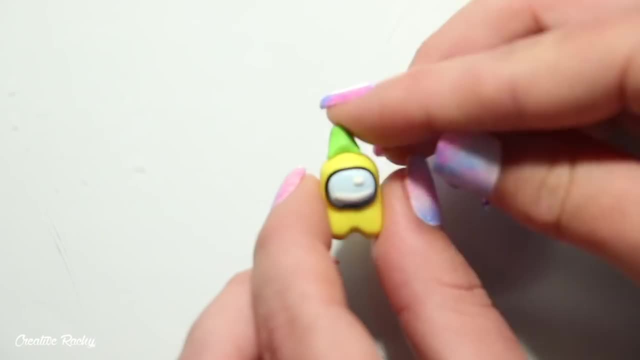 For the eye. I attached on a small ball of white clay and then I rolled a thin coil of black clay to create a rim- again Kind of the same method as I have for the crewmates, just wrapping it around the outside and cutting off the excess. 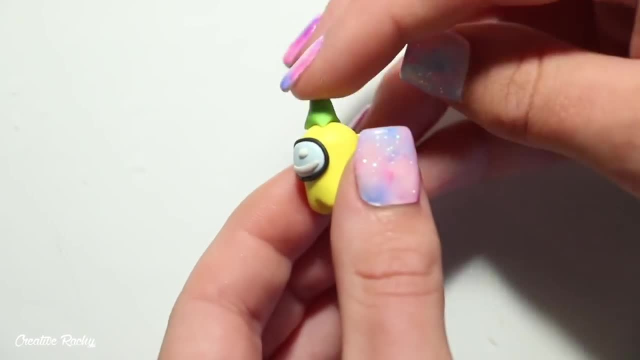 So there you have it. I hope you enjoyed this video. If you have any questions, feel free to leave them in the comments below, And I'll see you in the next one. Bye, Bye, Bye, Bye, Bye, Bye. 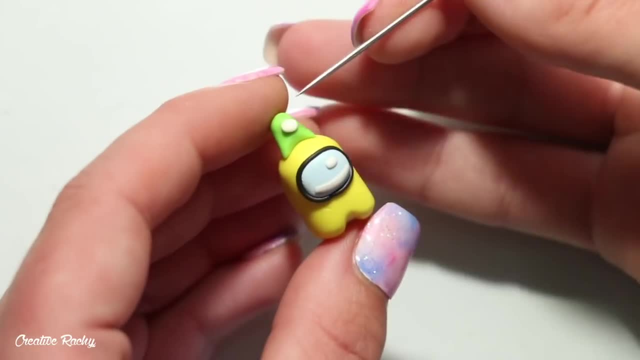 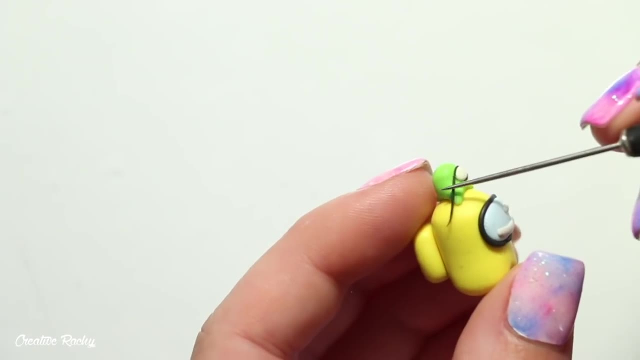 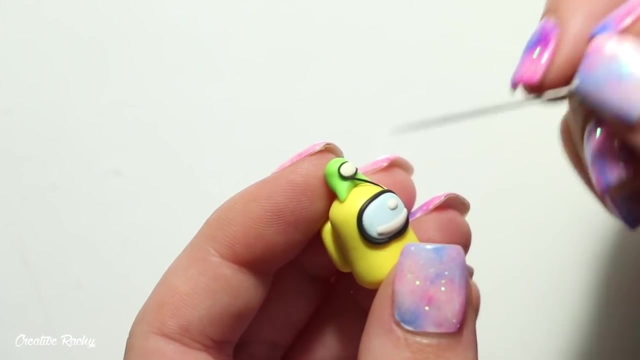 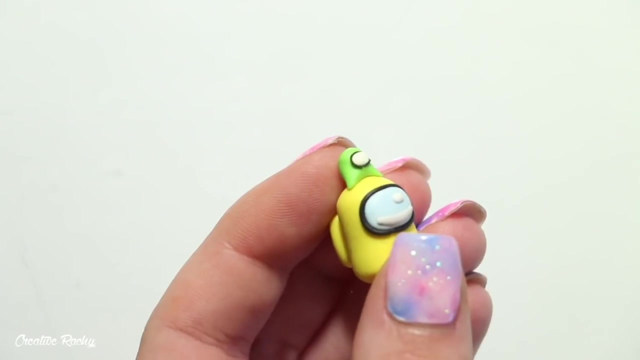 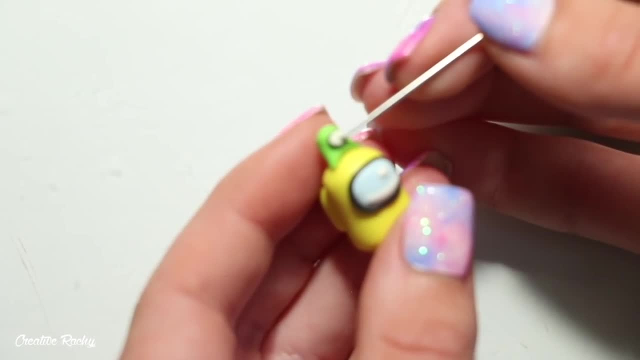 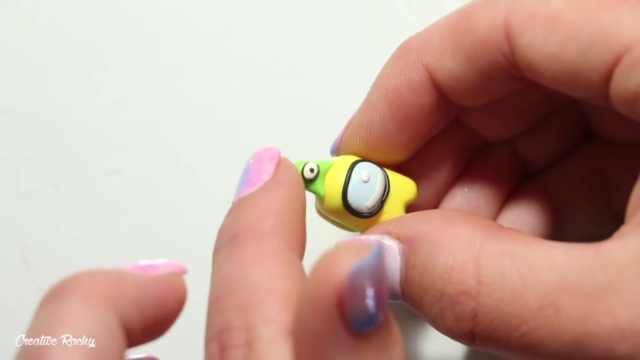 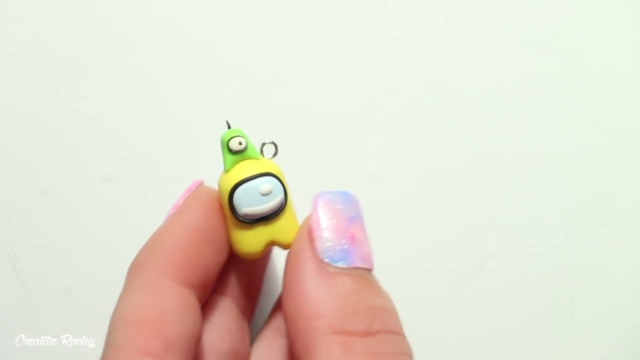 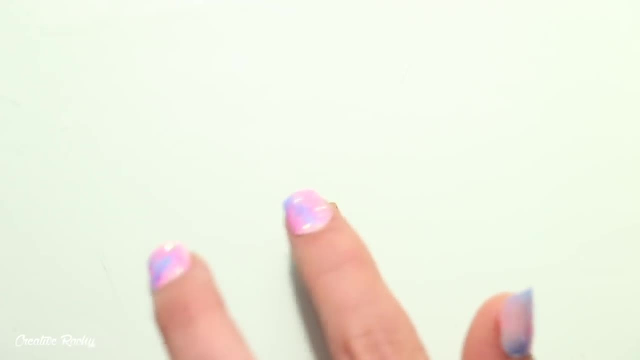 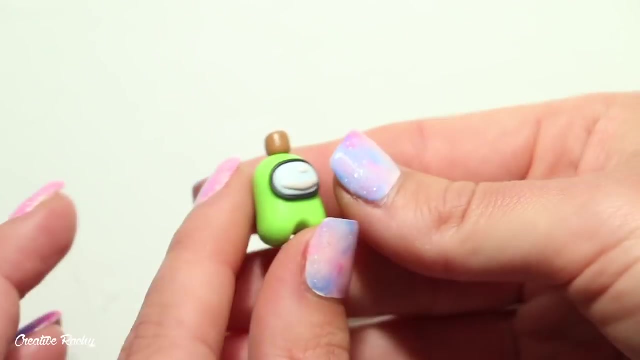 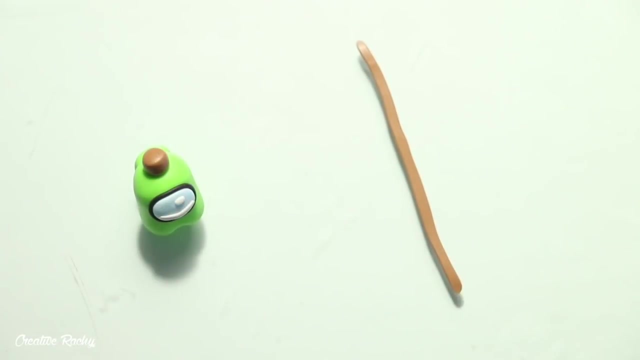 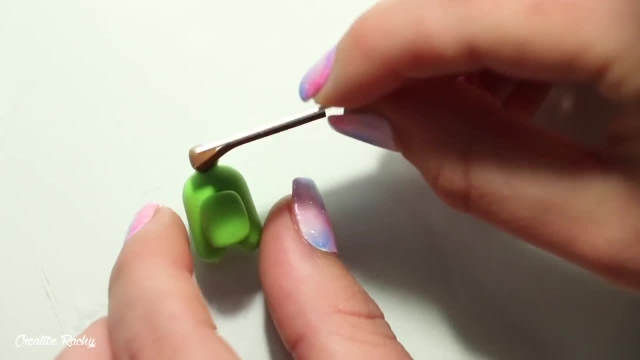 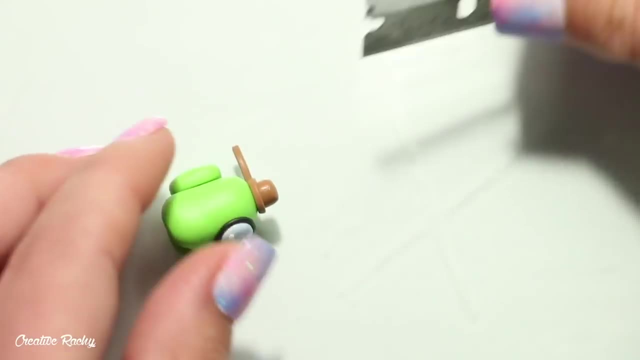 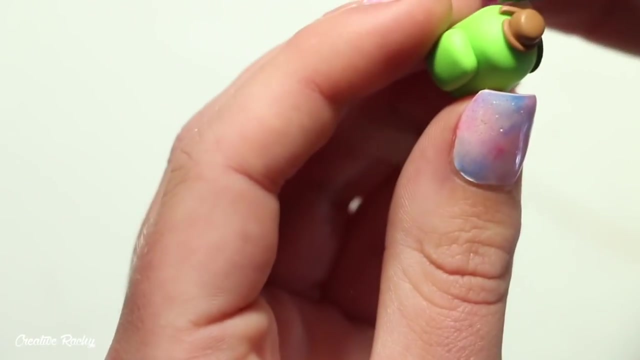 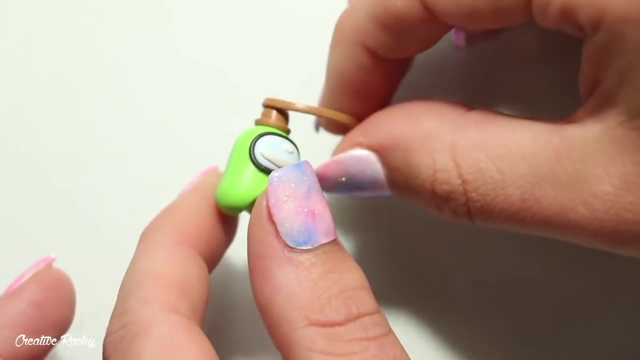 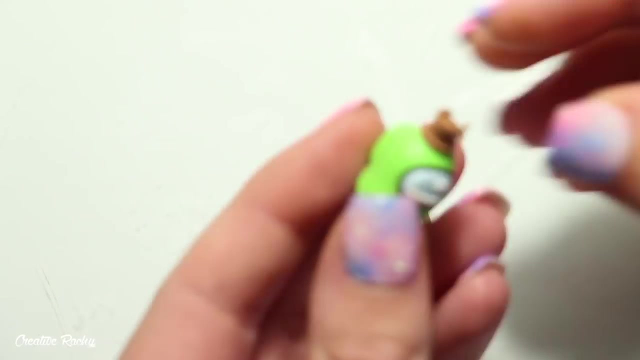 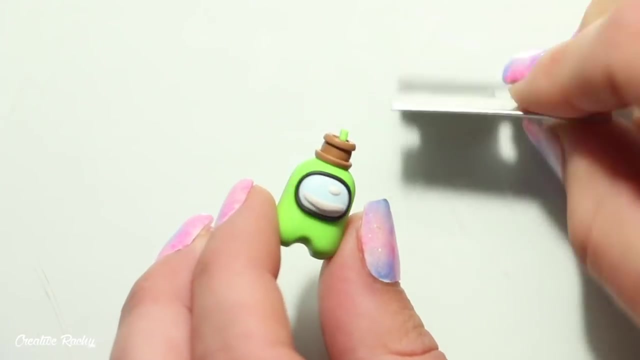 nice and neat. Then begin wrapping these pieces of clay around the pot for the rims. Add one to the top and one to the bottom of the cylinder and just cut away any excess clay. Next add a little stem with some green clay and also add some leaves on either side. 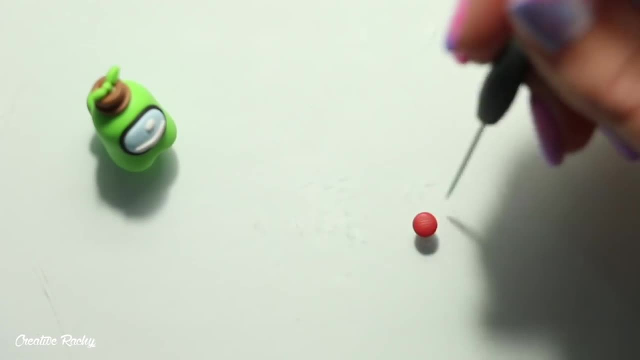 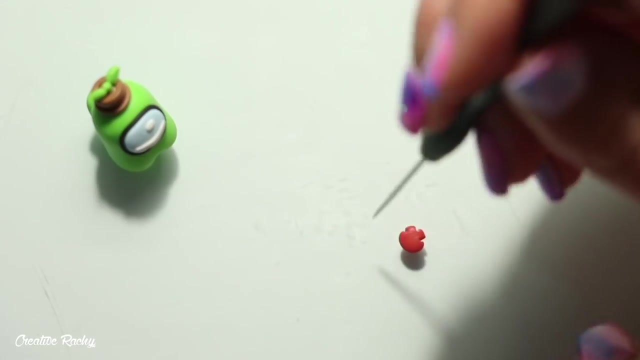 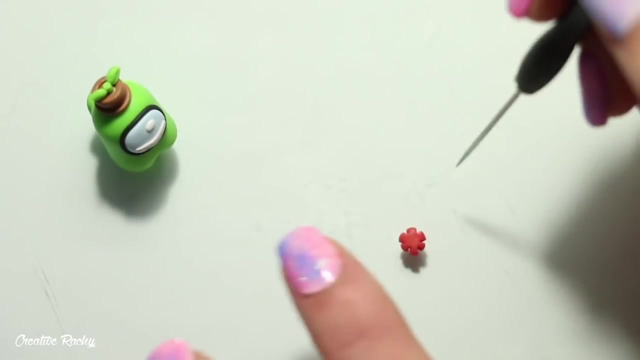 To make the little flower, I flattened down a ball of red clay and then I just used my needle tool to go around the outside and add some little indents to the bottom of the pot To create the petals. I made an indent in the center with one of my ball tools and then I 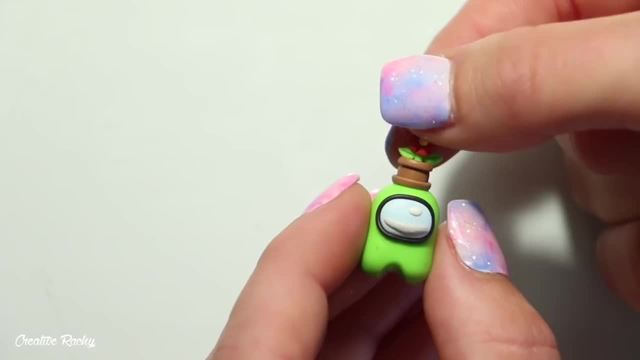 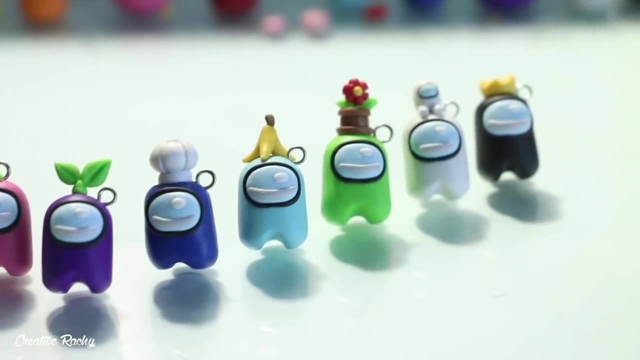 positioned in a small ball of yellow clay. I then attached the flower to the stem and I added an eye pin to make it into a charm. Here's what all my crewmates looked like together before I went ahead and baked them. After baking, I took some super glue and I used this to secure the eye pins. so that they wouldn't break. I then used a little bit of glue to secure the eye pins so that they wouldn't break. I then used a little bit of glue to secure the eye pins so that they wouldn't break. I then used a little bit of glue to secure the eye pins so that they wouldn't fall out.